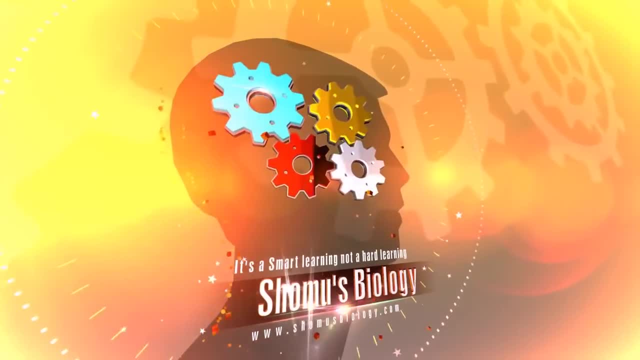 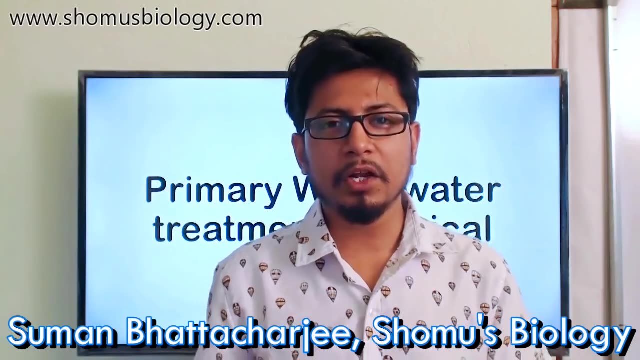 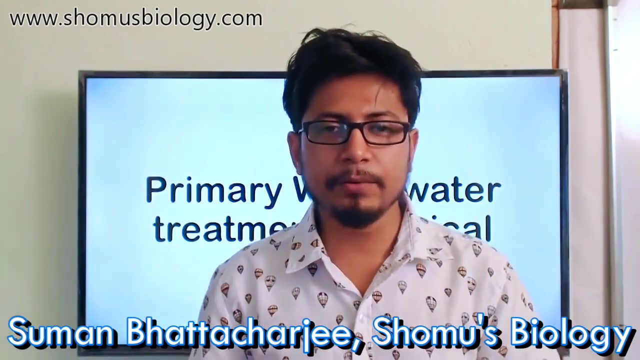 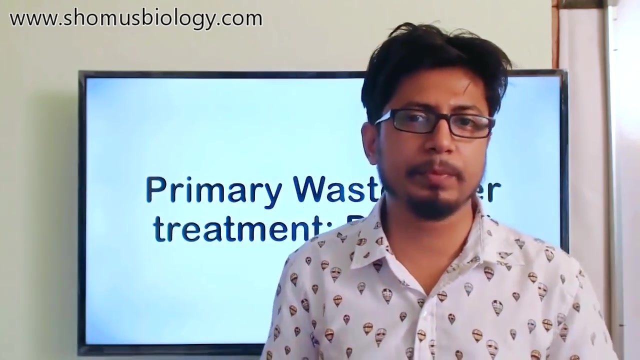 Hello friends, welcome back to another video tutorial from Shamos Biology and we've been talking about the wastewater treatment process and we've seen the overview of wastewater treatment in the last video lecture and we also talked about the preliminary wastewater treatment and we know that after the preliminary wastewater treatment, the water, the wastewater, moves to 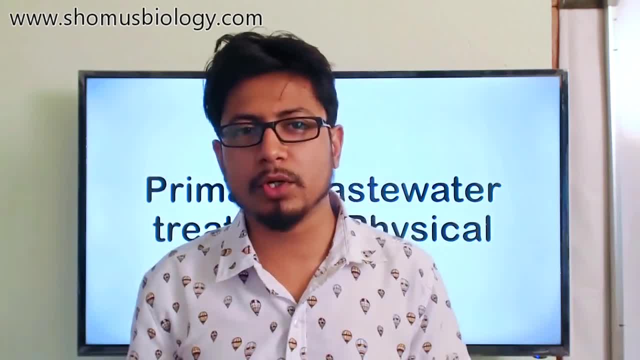 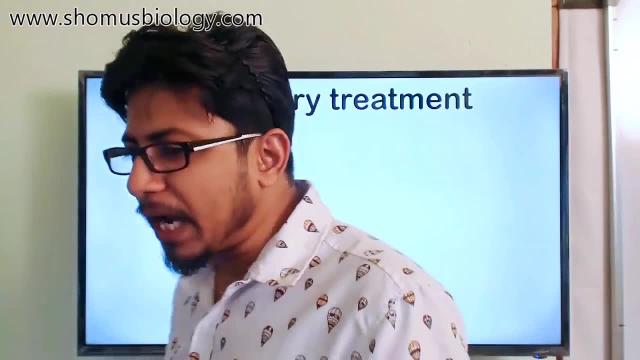 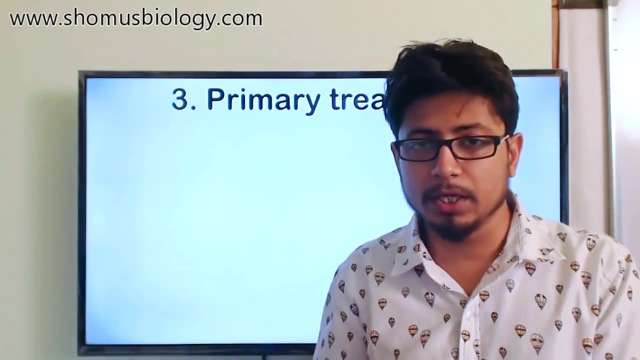 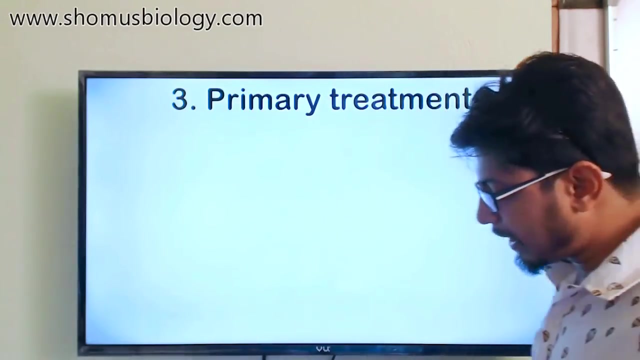 the primary wastewater treatment. So now we are going to talk about primary wastewater treatment and what happens in the primary wastewater treatment process. In the primary wastewater treatment it's a physical method of wastewater treatment separation. That means we are separating solids from the wastewater with physical barriers, And in this case, what kind of physical barriers we use? We do the same kind of physical barrier mediated separation of large solids from the wastewater using 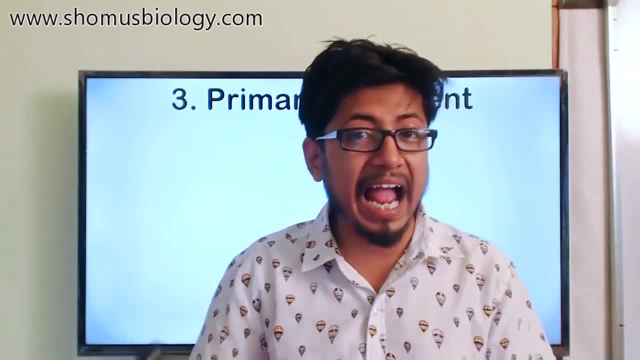 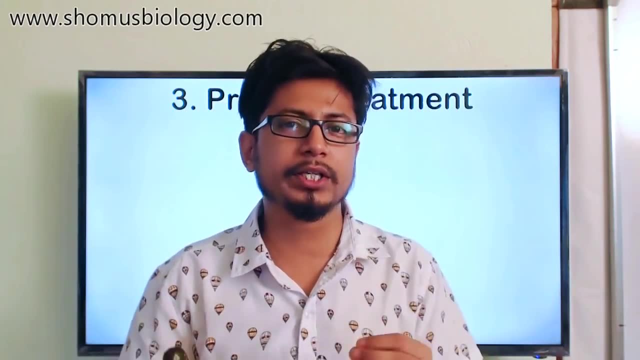 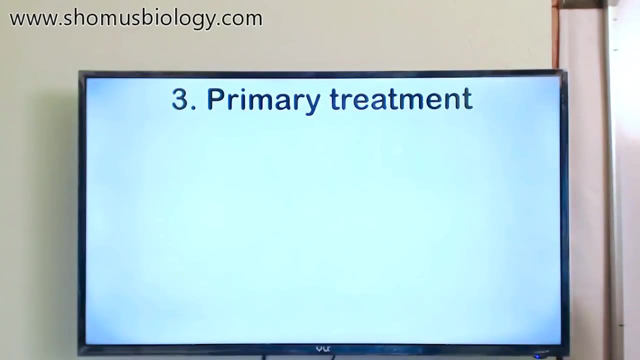 preliminary treatment. But the major difference between a preliminary wastewater treatment and a primary wastewater treatment is in the primary wastewater treatment we simply use a gravitational force for the solids to settle down to the bottom of the settling tanks or clarified tanks in the primary wastewater treatment. So approximately 25 to 50% of all incoming biological oxygen demand, 50% to 70% of the total suspended solids and 65% of the total suspended solids. 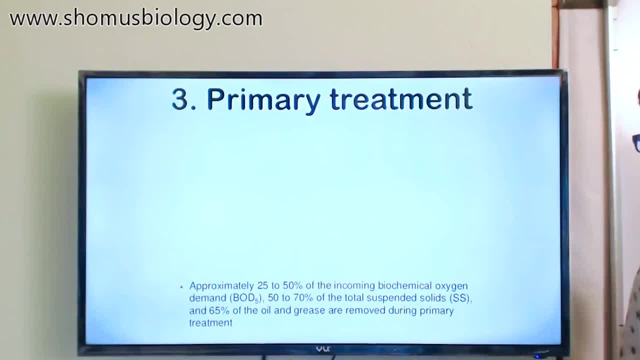 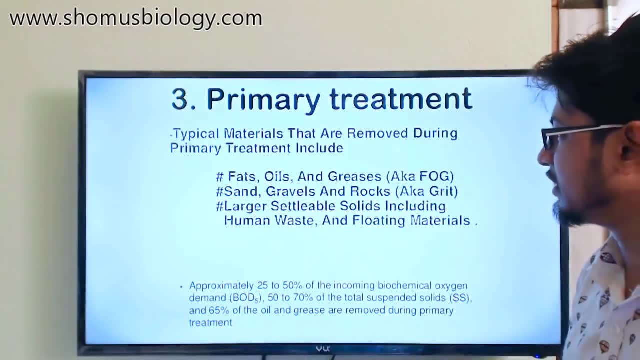 are removed during the primary wastewater treatment. So this is our motto, And the materials we generally separate with primary wastewater treatment is fat, oils and grease, which we know as a FOG form, sand, gravels and rocks, aka grit, and larger settlement solids, including human waste and floating materials. These are all are getting filtered from the wastewater And this 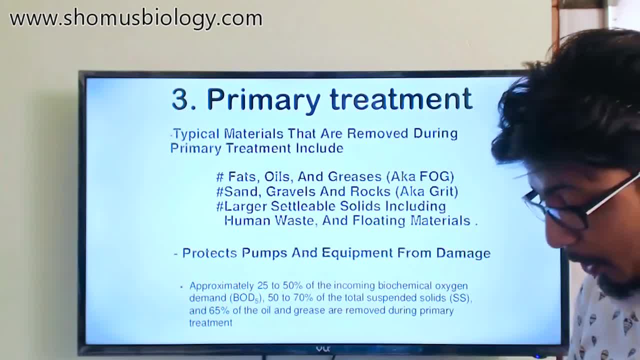 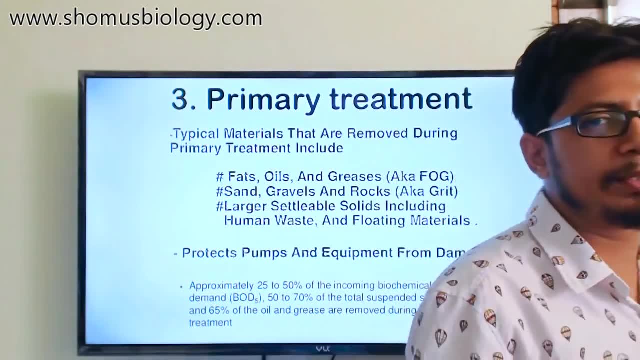 primary treatment protects pumps and equipments from damage, because the moment the water will move to the next secondary treatment, tertiary treatment, the machines may get damaged if the solid materials are still present in the wastewater. So it's very important to reduce them and remove them. That's what we are doing with the 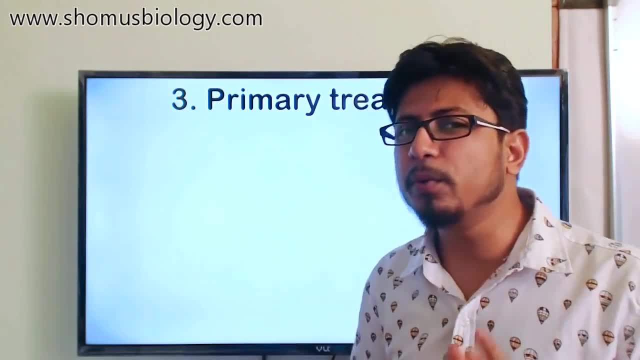 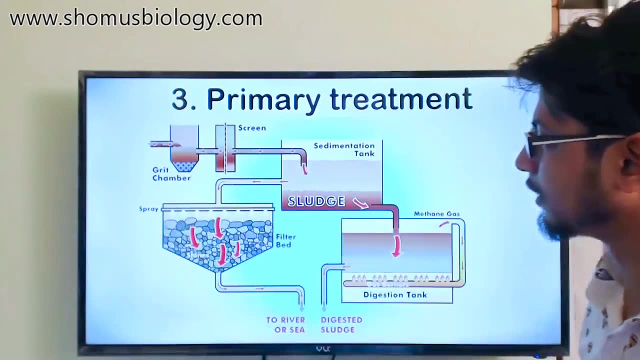 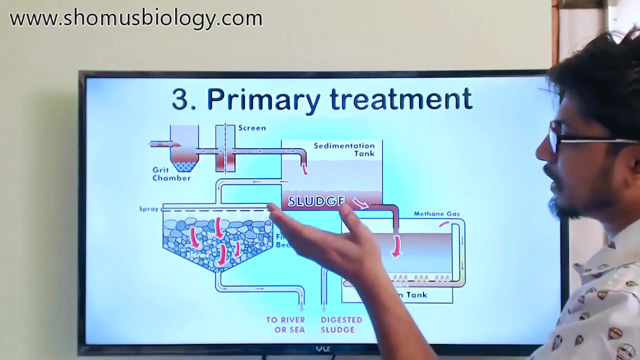 help of primary wastewater treatment. So the major equipment of primary wastewater treatment is a big tank known as primary settlement tank of the wastewater. You can see in this picture is the sedimentation tank, known as the primary sedimentation tank. in this picture you can see two different lines. if I draw a line from this middle one, 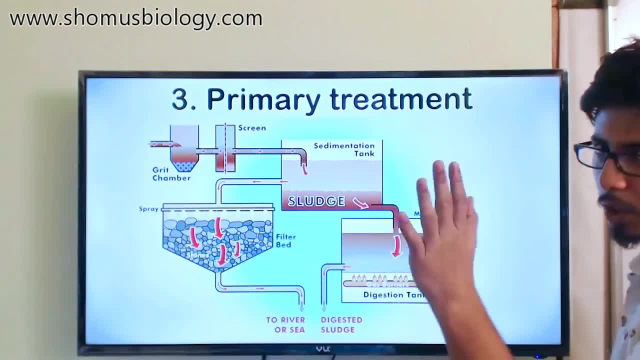 picture is on top, another is in the bottom. the things present in the bottom is not our concern because things in the bottom are secondary waste water treatment. we will talk about that in the next video. but the picture in top is what works in the primary waste water treatment. so water comes in through the 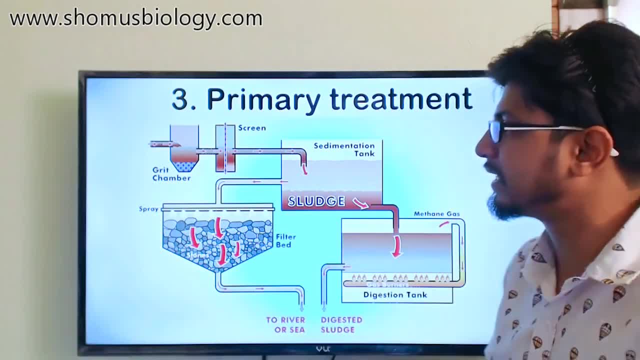 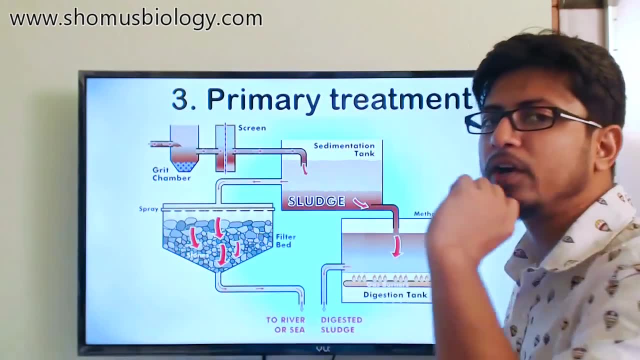 grid chamber generally. grid chamber is a part of preliminary waste water treatment and screeners, who generally separates larger solid particles. so we know this is the part of the preliminary treatment and we have already checked that part in the last video. if you haven't seen that, please watch that video so that you can. 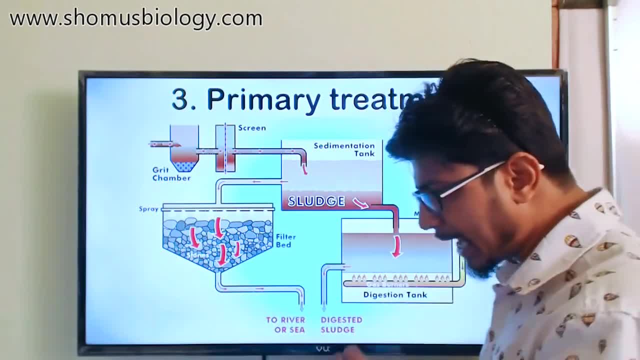 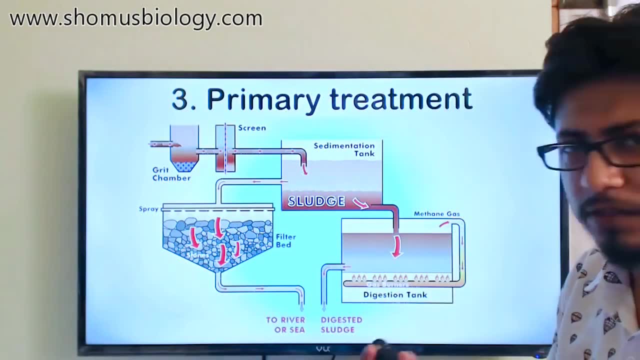 make more sense about this video. so the water now comes in. it carries dissolved solids. it carries some solid particles which are not that big, but, yes, rock, gravels and all these sands. everything is there. so what we need to do is use this huge sedimentation tank. we call it primary. 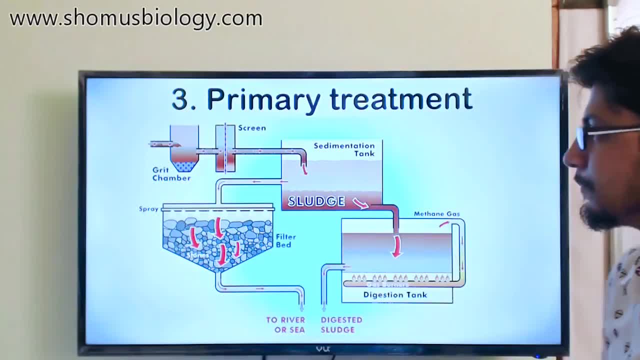 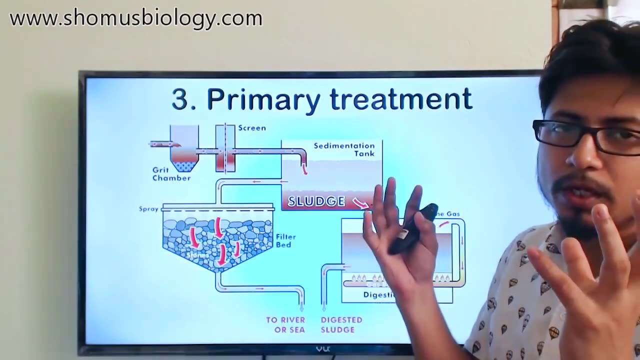 sedimentation tank or primary clarifier tank, this primary sedimentation tank, where all this water filled with waste water, filled with the solids are placed, and in the sedimentation tank, what happens? that those all solids start to settle down to the bottom of this tank. and as it's settling down to the bottom of the tank, 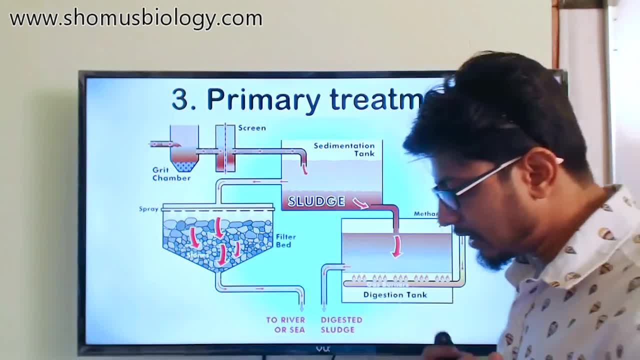 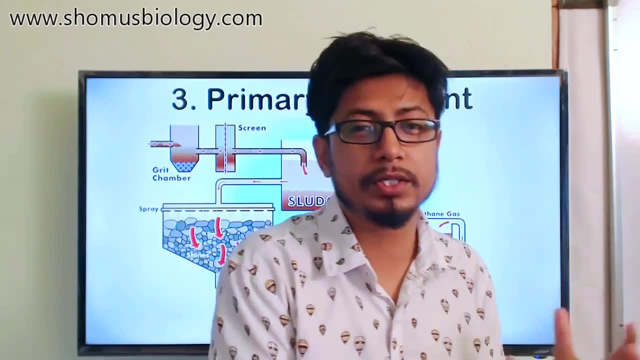 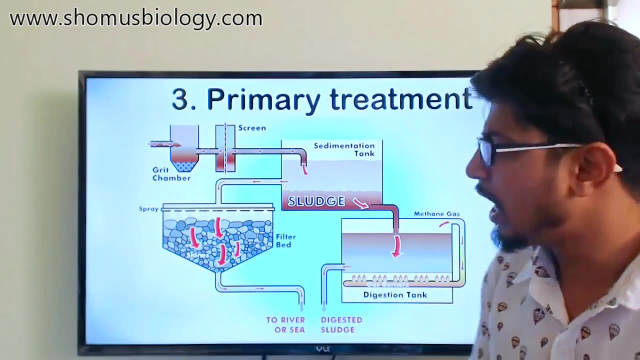 we are calling it as a sludge. the sludge is is a name for any other large components, large or solid components in the wastewater which is not floating in the water which is being settled to the bottom because of its higher weight in this gravitational force is getting settled to the bottom. now the question is: for this settlement we need 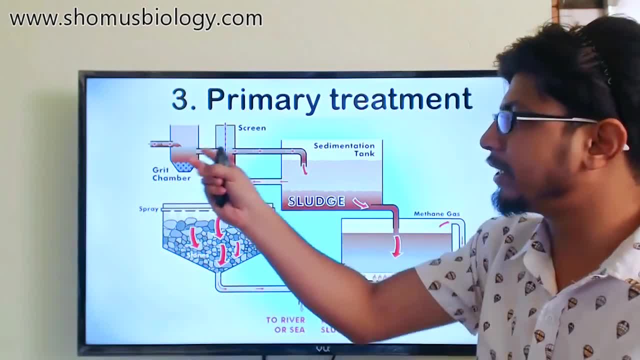 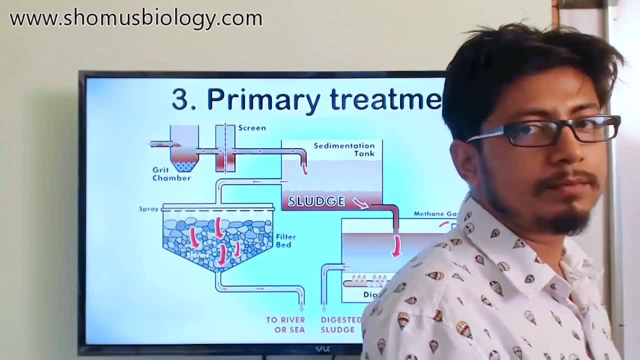 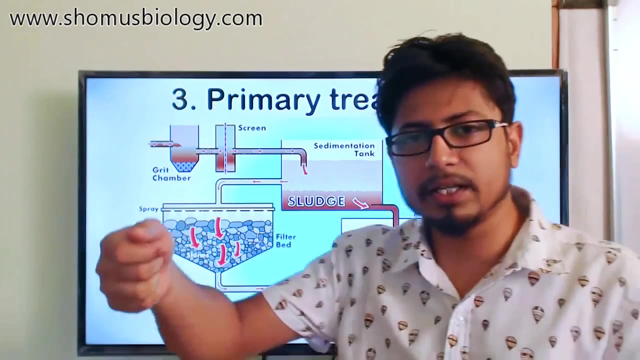 to reduce the flow of water because, till the point of this preliminary treatment, the water was continuously flowing. now, in this case, to prevent the water to flow less, what we can do simply, we use this large tanks and the water flow is regulated. we slow down the water and we allow the water to settle down. 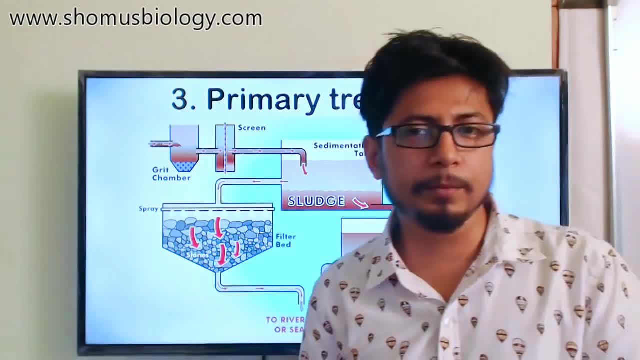 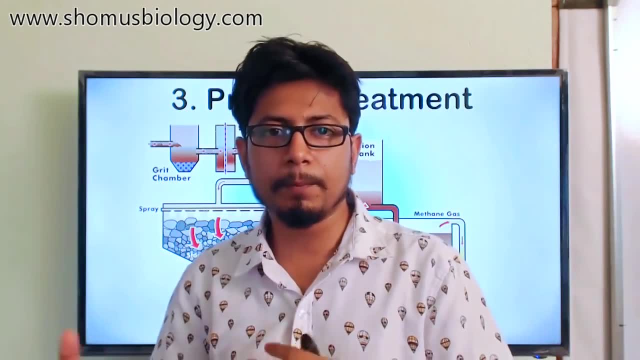 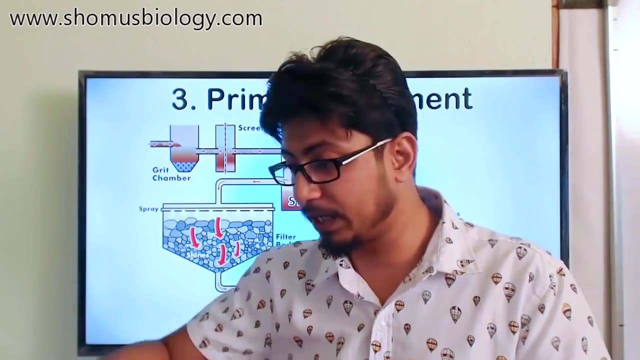 ok, because during the process of connection to you, as well as preliminary treatment, water was flowing, but at this point we are slowing the rate, so we measured this as a flow per minute. that means the, let's say if you drop something in this water and what distance it will travel per minute, or what distance it will travel per second. 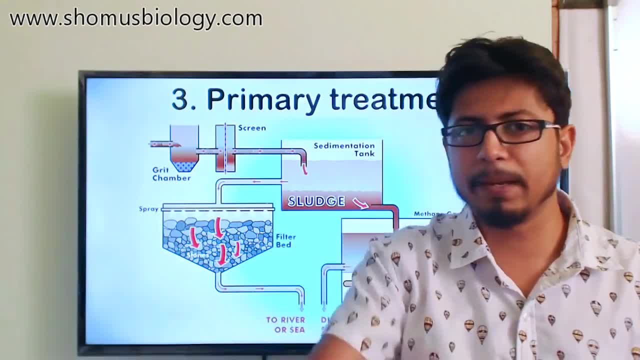 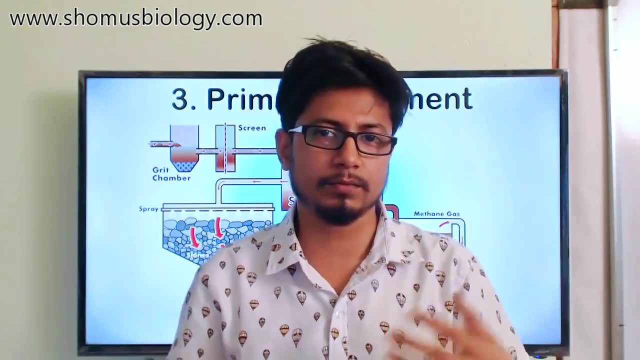 that's how you measure the flow of water. so if you put a solid, let's say a paper, you just put it into the water. it only moves 10 feet in a minute. so you say the flow rate of the water is 10 feet per minute. 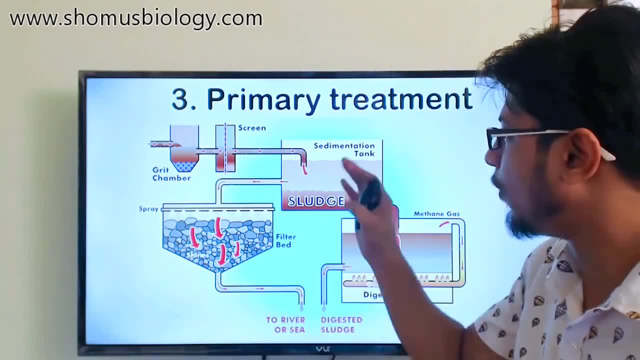 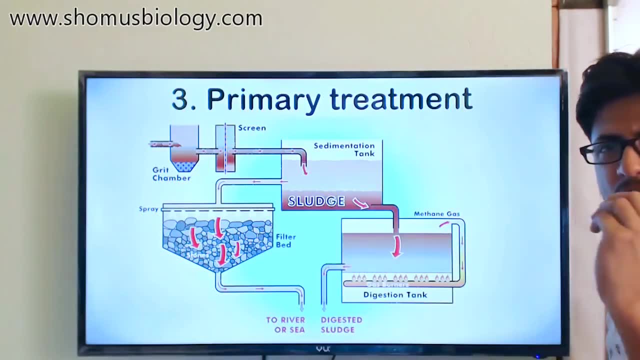 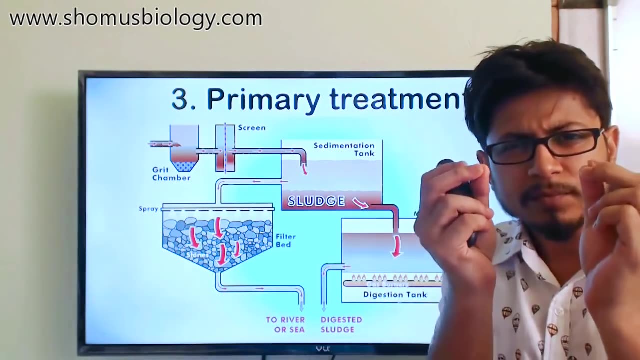 so this is the kind of situation is. so we reduce the flow of water in the sedimentation tank because the more we reduce the flow, the better sedimentation we can achieve. so whatever large solid particles settle down to the bottom, known as a sludge, and there are very few things what we can say, that smaller oil, like components which are floating on the top. 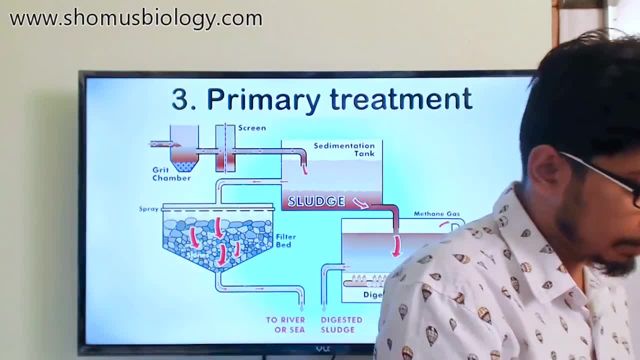 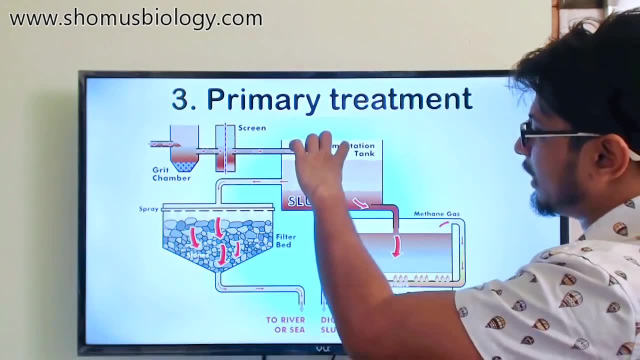 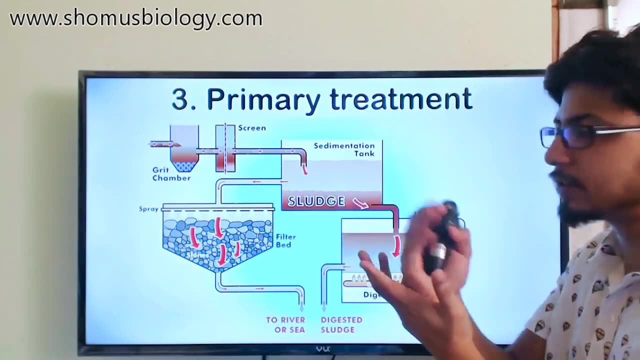 grease floating on the top because they cannot settle down to the bottom. so we need to use two types of schemas to separate these things. you know one. so in the sedimentation tank we have a rotor. in the rotor we have two different arm like structure: one on the top connecting to the surface of the arm. 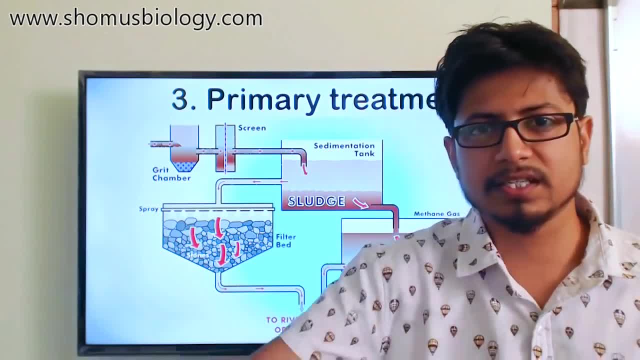 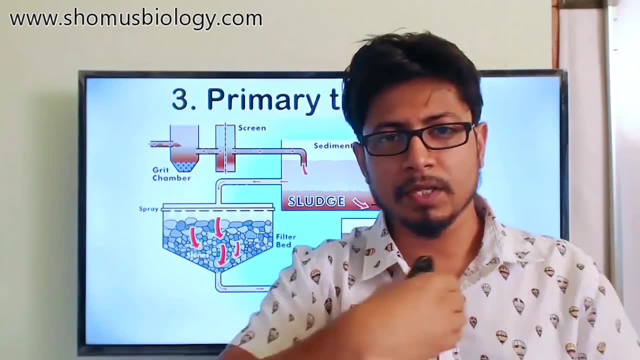 and one on the bottom. the bottom one is scrapping all the sludge and collecting them to the bottom, and the arm that is present on the top is actually separating all those- what I can say, the grease, oils, oil, like components, separating from one another. 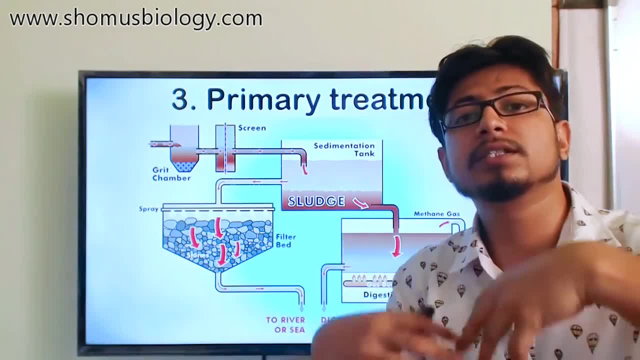 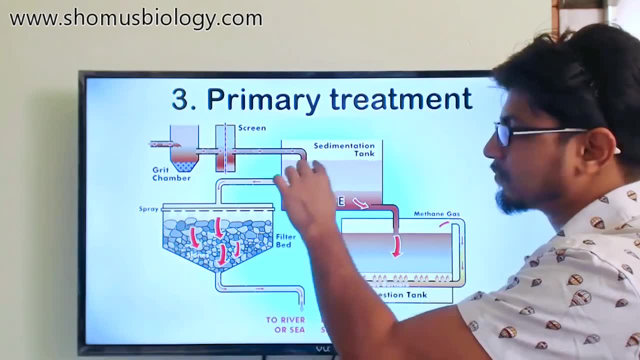 we call it scum. so there are two types of wastes that are produced from this primary sediment tank. one is the scum, which are grease and oil droplets which are formed on the top, so scum settlement, and then the large, very solid particles settling down to the bottom, known as the sludge. 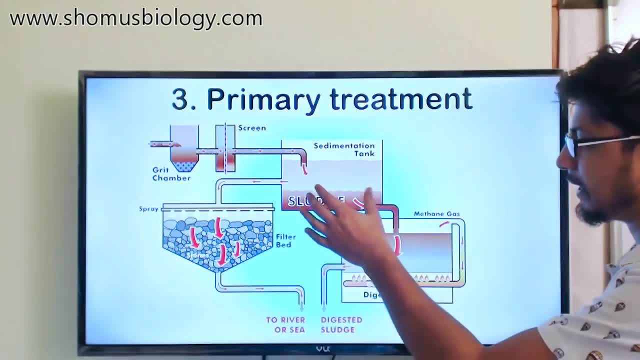 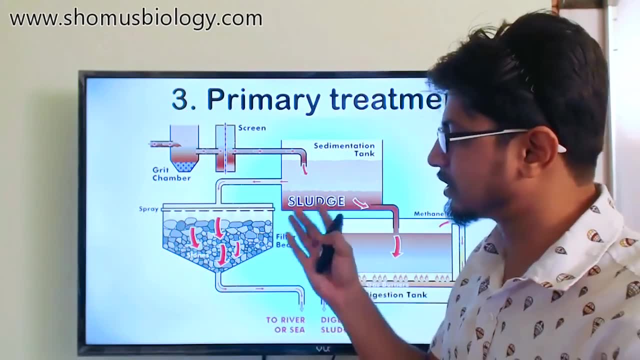 we separate them as usual. so the sludge, once separated, is transported to a sludge handling facility afterwards, and the effluent, which is separated from the sludge and scum, is transported to the next stage of the waste water treatment, which is the secondary waste water treatment. 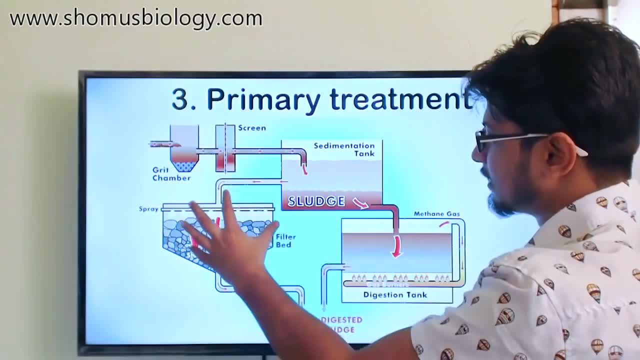 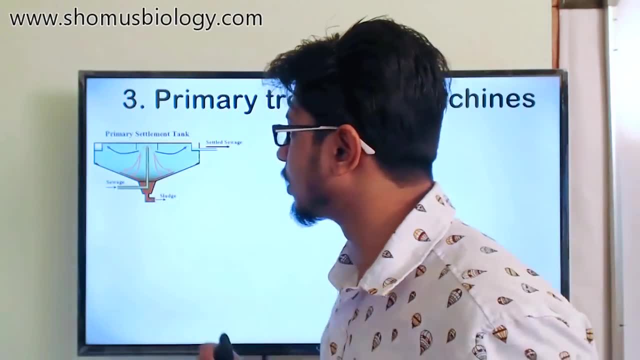 which we will see in the next video. so this is preliminary and this is secondary, and in the middle we have the primary waste water treatment. so if you see the machines that are involved, this is what we are talking about. this is the rotol that is in place. 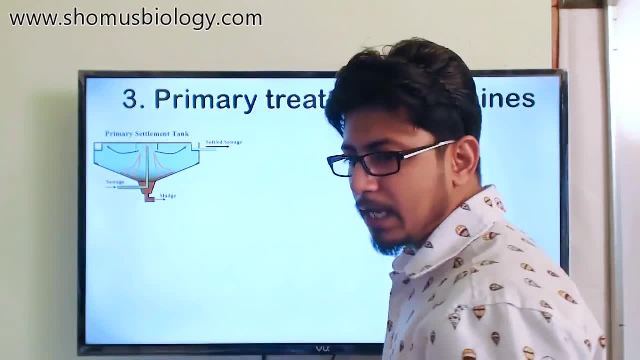 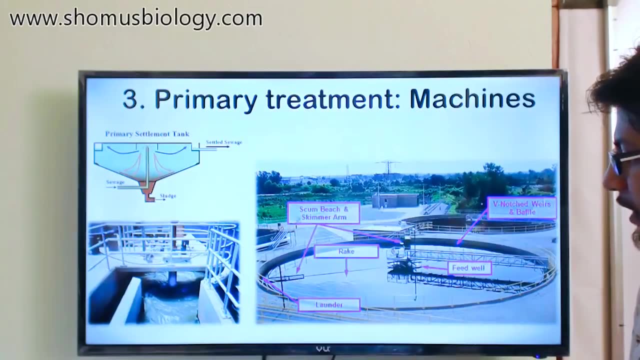 and we have the sludge and we have the scum. so if you look at this picture, this is how it looks like. this is the large tank, primary settlement tank. you can see this picture here as well: large primary settlement tank, and the beauty about this tank is: 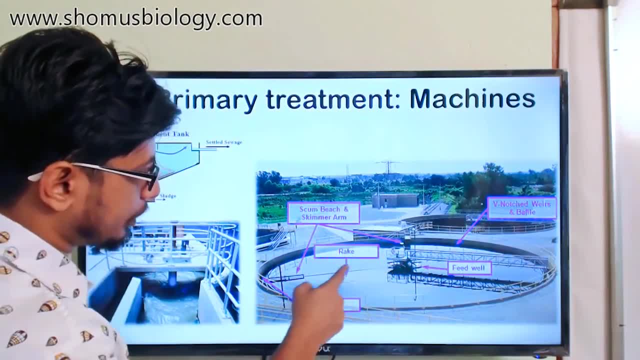 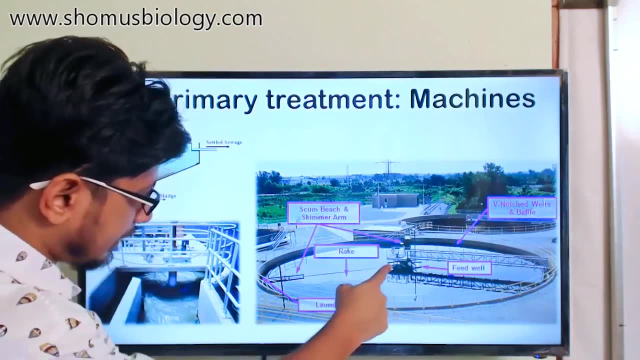 is that, if you look at this, this tank contains these two regions. you know one. this is the bridge where the people can go and can check whether everything is okay or not. center is the motto and this is the red. as I said, there is a rake to separate the scum. 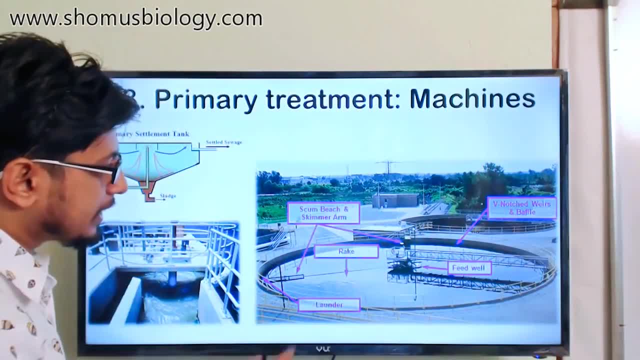 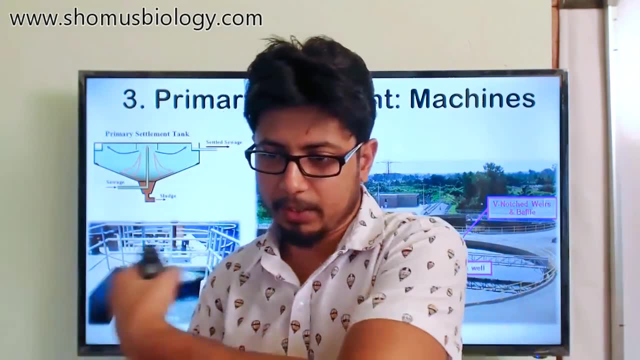 and also a rake in the bottom to separate the sludge so you can see scum match back. this is known as schemer arm. schemer is that kind of mechanical structure that will scheme and separate all those geese and floating oil materials from the top. 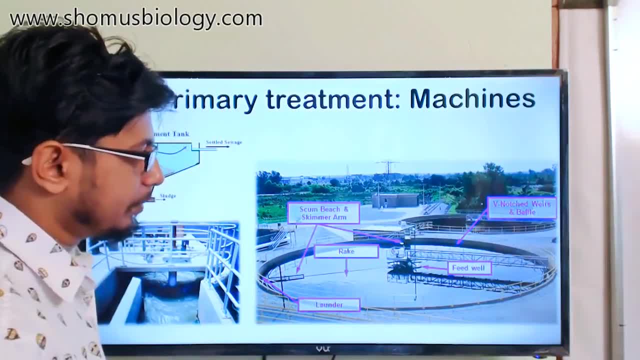 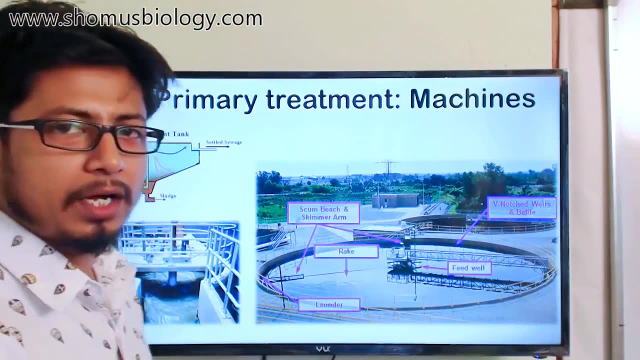 and in the bottom also, there is also another schemer which is not visible in this picture, but that's the thing you know. this thing continues rotating. so if you look at the top view model, it looks like a clock. the arm of the clock is moving like a schemer. 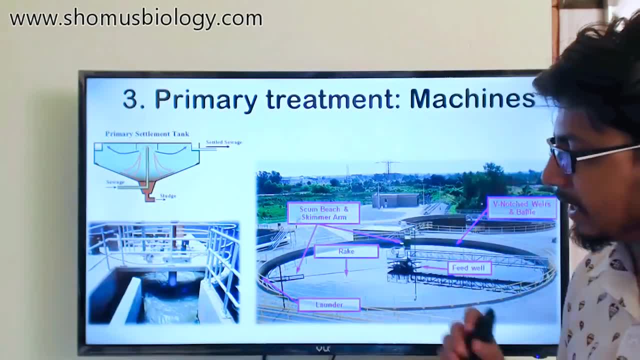 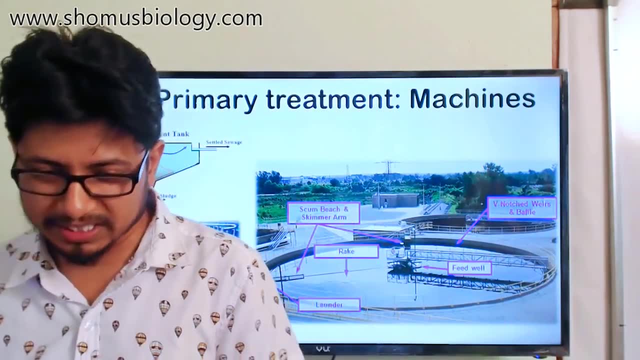 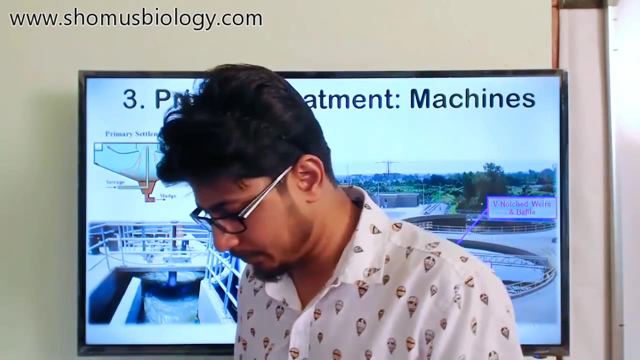 separating all those scums on the top layer and sludge in the bottom layer. okay, so that's how it's- separating scums and sludge from the wastewater- and that's our motto in the primary treatment: to separate any solid material that is present as much as we can. 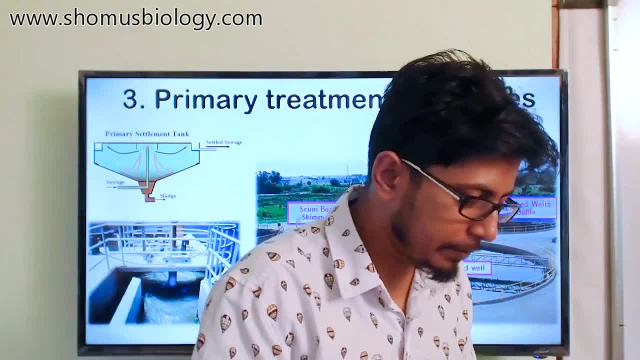 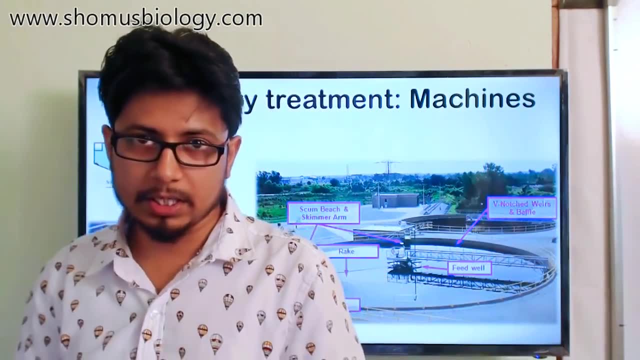 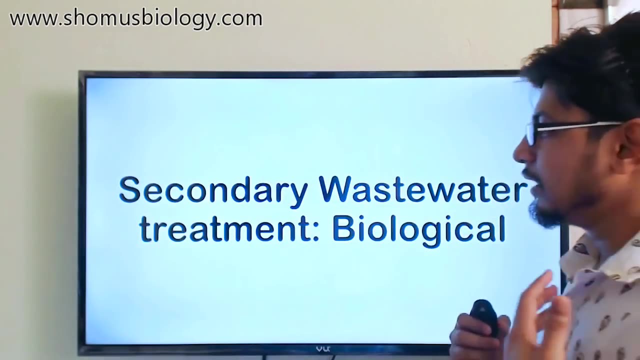 and we use gravitational force for the solids to be settled down, because if we fail to do so, if this solid particle still remains in the water, that may damage the further process of wastewater treatment downstream. okay, so that's regarding the primary wastewater treatment. now, in the next video, we will be talking about